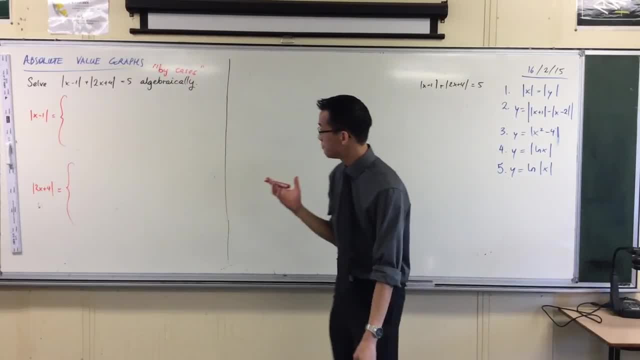 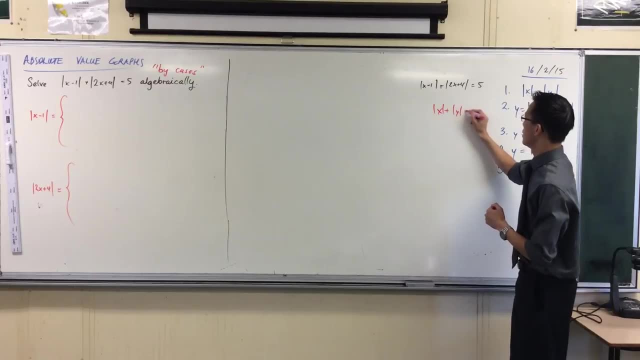 So you might hear that phrase sometimes, and this is what it's referring to. Here's the way I'm going to break it down. Do you remember? at the start of the lesson, I showed you this, Whoops? I showed you this right. 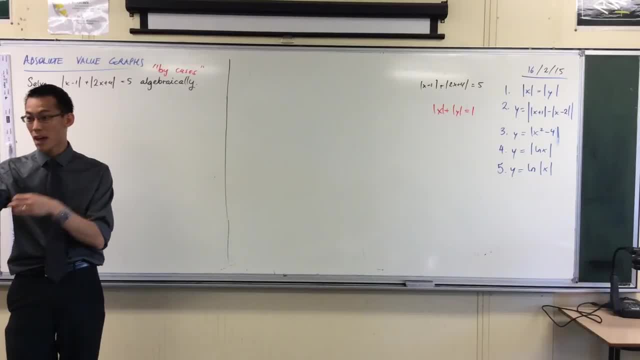 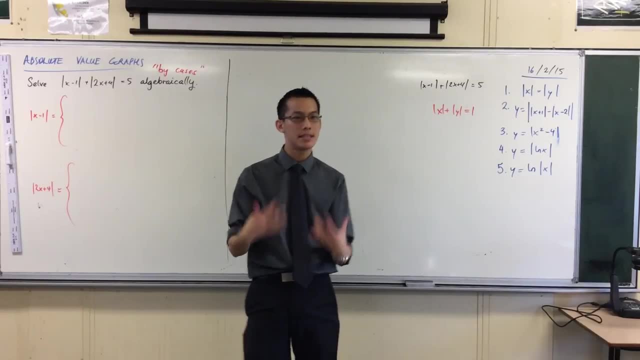 So I said: look, the absolute value of x is equal to this sometimes and this other times. And then I said: y, the absolute value of y is equal to this sometimes and this other times. I'm going to replay exactly the same scenario. 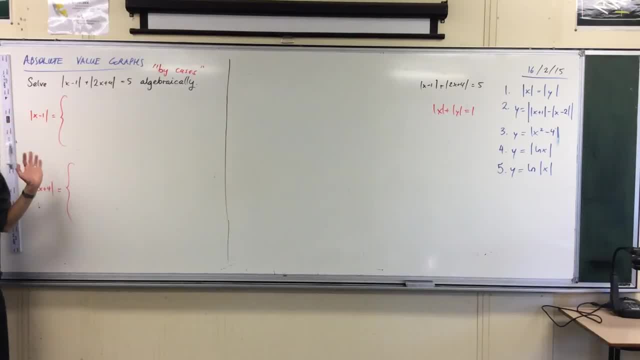 But I'm going to replay with these two, okay, And that's going to. once I do that, that will give me the cases that I will then solve. Okay, so watch. Absolute value of x minus 1, okay, Sometimes it's equal to this. 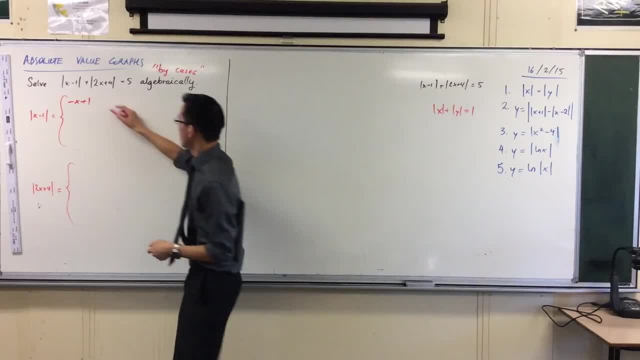 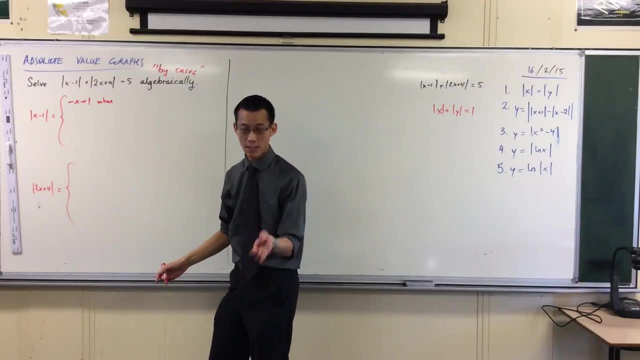 Okay. so this is me saying the negative case. okay. So I say when that thing inside the brackets is negative, That's when you slap a minus sign on it, When x minus 1 is negative, okay. Okay, It's a bit of an awkward way to say it. 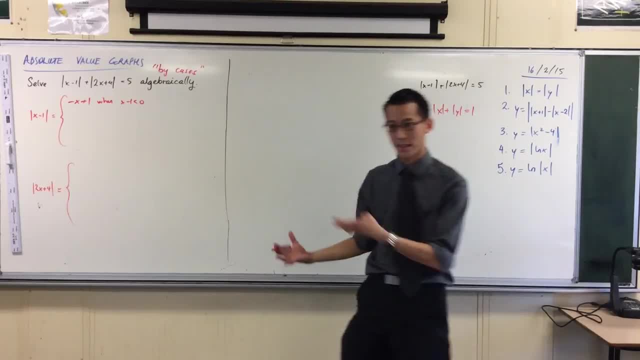 I would like just a domain that just says x is greater than this or less than this, and that's fine. So I'm just going to muck around with this a little bit: x is less than 1.. There you go. 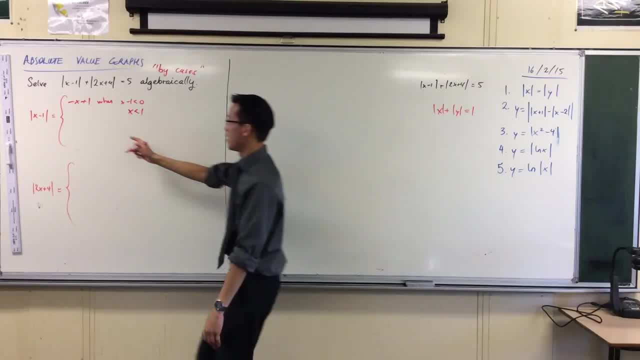 That's where that's the condition I apply for. when this is true, okay. Alternatively, I'm just equal to this when x minus 1 is positive or inclusive of 0. It doesn't matter, as you can see, right. 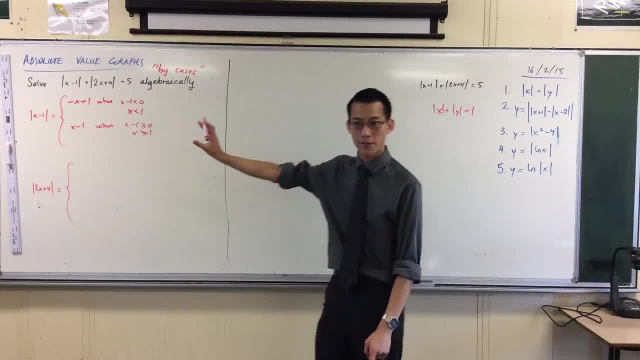 So this is when x is greater than or equal to 1.. Okay, great, I have two cases. I have two cases for that guy, Two cases. When you come down to here, you replay it in exactly the same way. 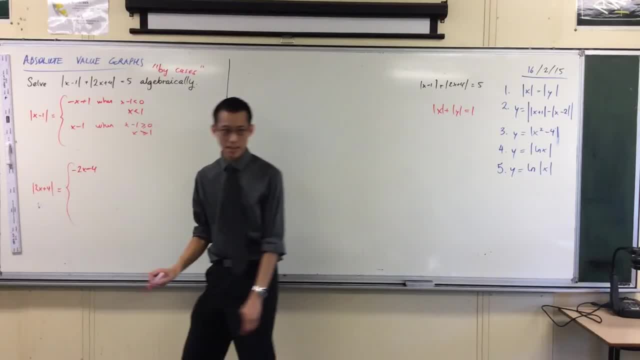 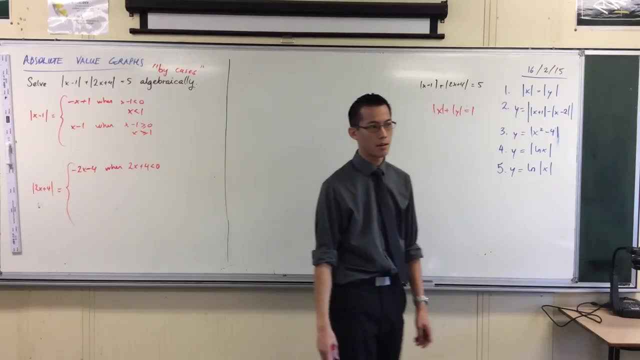 I'm going to be equal to the negative case minus 2x minus 4, when that thing inside the brackets is less than 0.. Okay, Now you will start to get to the point where you do not have to go through all of these lines of working. 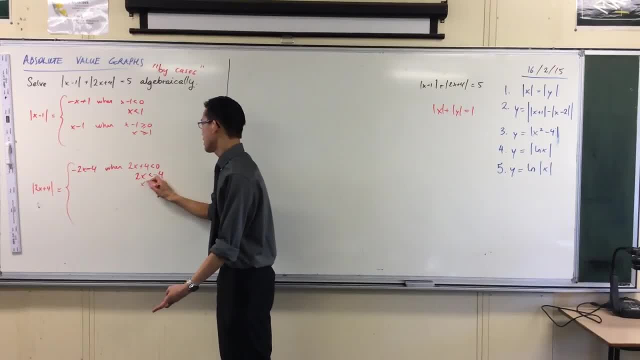 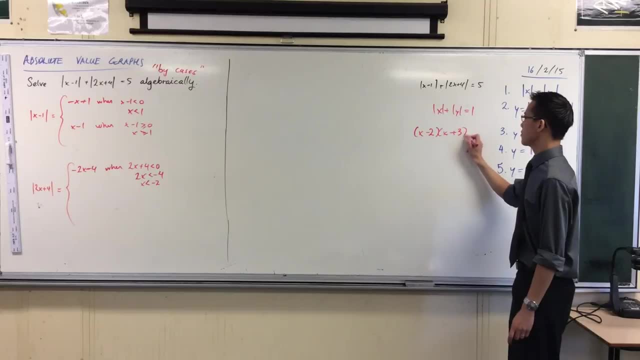 where you'll be able to see right away: oh, it's x is less than negative. 2, right, In a similar way to. So if you guys see this, you don't um and ah and think: ooh, what are the 0s? 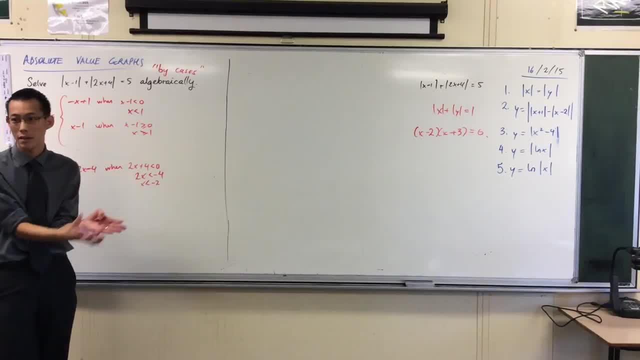 You just read them off. You say negative 3 and 2, because you've seen these so many times, You'll start to do the same thing with this. It's a very similar kind of situation. I'm going to take a bit of a shortcut and say: okay, once I know where the negative case is true. 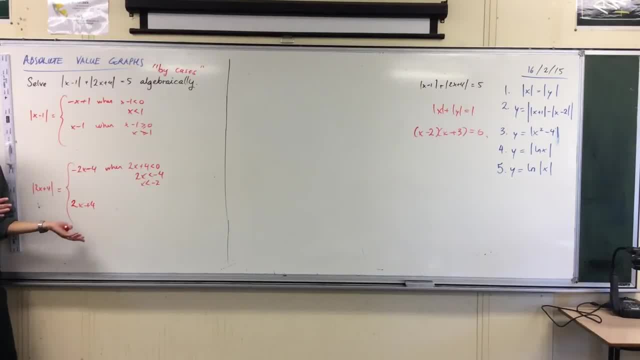 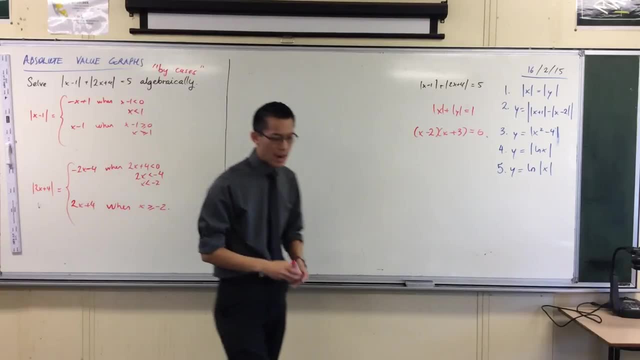 I also right away know where the positive case is true, because it's just the other side of the inequality. So it's equal to that when x is greater than or equal to negative 2.. Okay Now, I said I was going to do this algebraically. 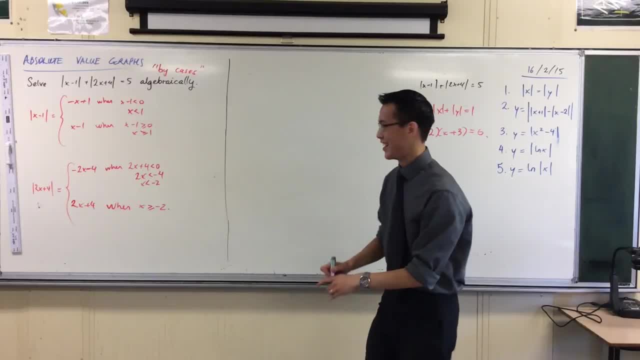 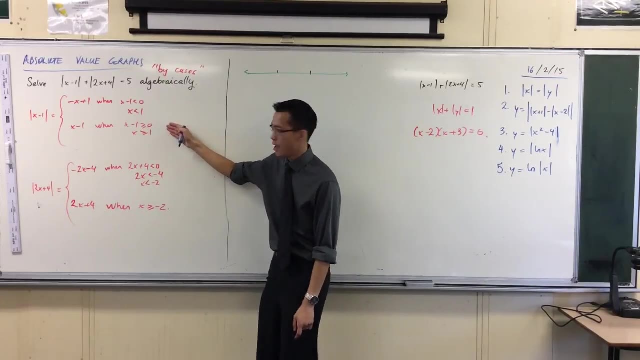 And um, I'm going to cheat just a little bit because I do have to um for myself. I have to draw a line, Okay, Um, why am I going to do this? right, You might think, oh, when I've got two cases here and two cases here, when I combine them. 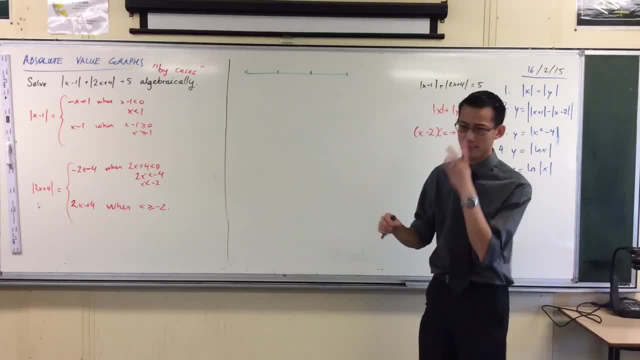 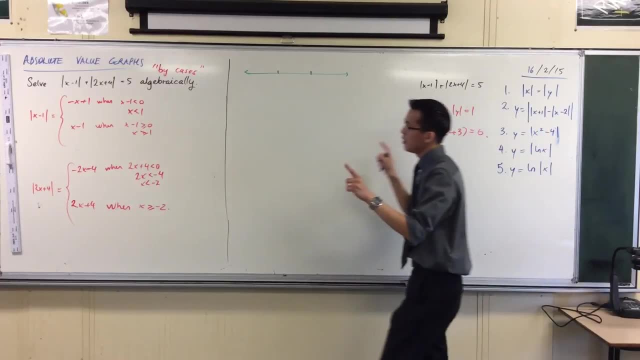 Shh, When I combine them, I should get four cases, Okay, Which is exactly what happened here, Right? But because all of this is just in one variable, right, It's just in x- You don't actually get four cases. 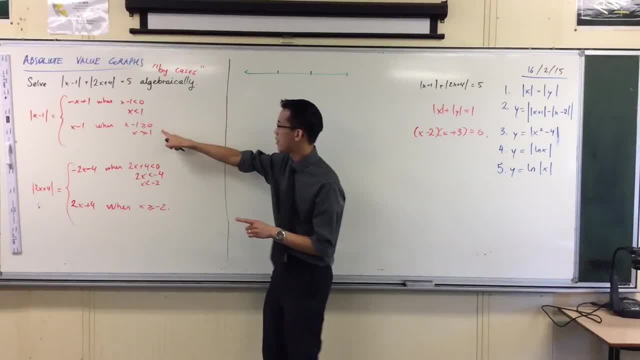 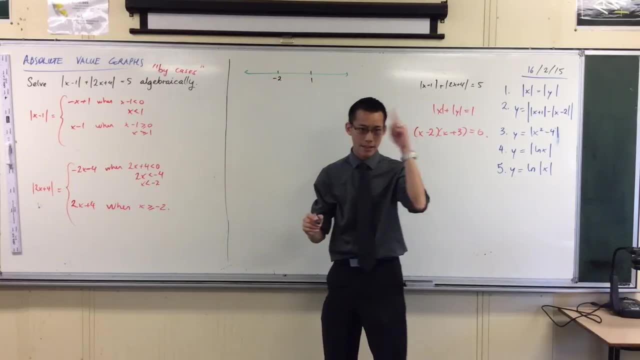 You only get three Watch. Uh, here are my boundaries. One is a boundary, Okay, And negative 2 is a boundary. So think about this, Okay, Think about what happens when x is less than or equal to negative 2.. 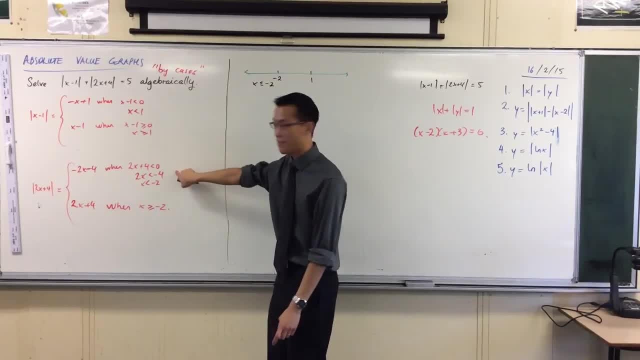 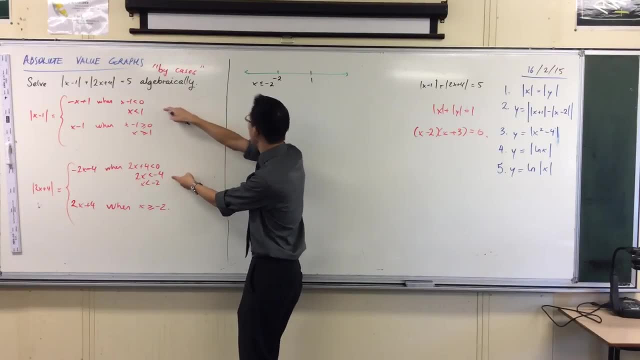 Right, Which of these cases are we in That one? Right, That's the case we're in. And then, which of these cases are we in? We're in this one. Okay, So I'm going to call that case one. 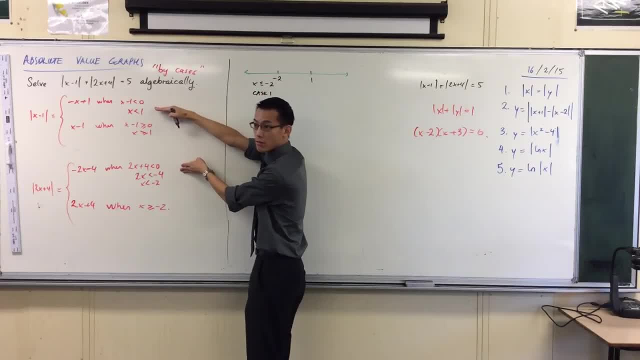 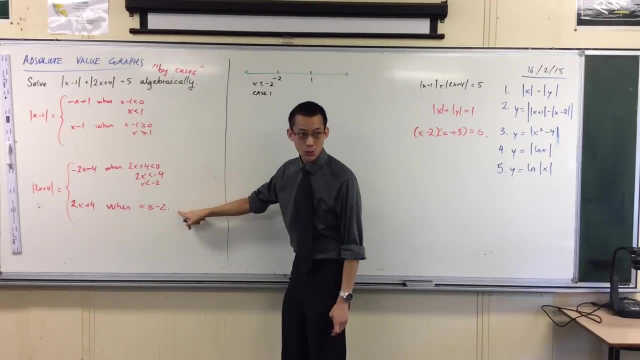 Okay, Case one is when I combine these two. Right, What about between negative 2 and 1?? Which case am I doing? Well, I'm greater than negative 2, so I'm this one, But I'm still less than 1.. 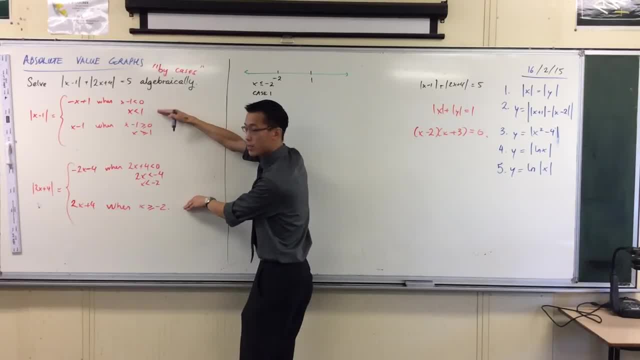 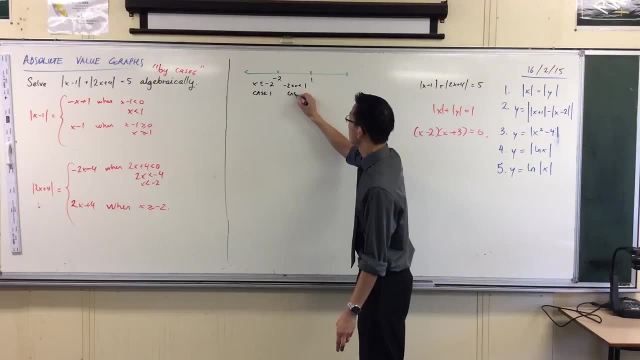 I'm still here, Right? So now I combine these two, Right? So, between these values, I'm going to call that case two. And then, lastly, you can see when x is greater than 1, I've already switched over to this one. 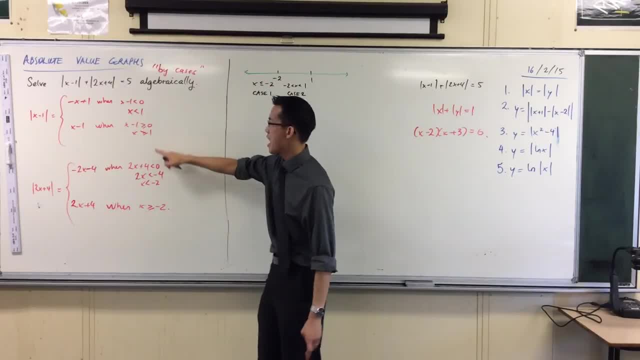 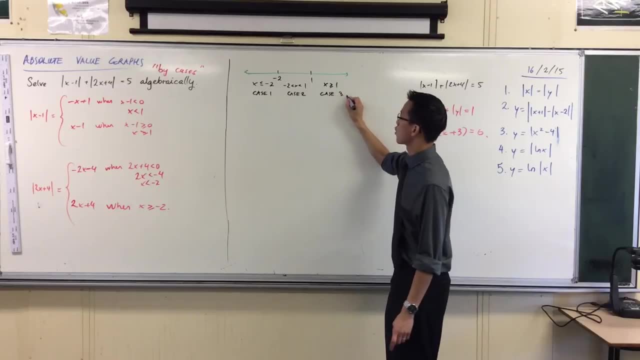 Right, Because I passed negative 2 over here, Right? So I'm in this one and now I've crossed over to this value, Right? So this is for. x is greater than or equal to 1.. I'm going to call that case three. 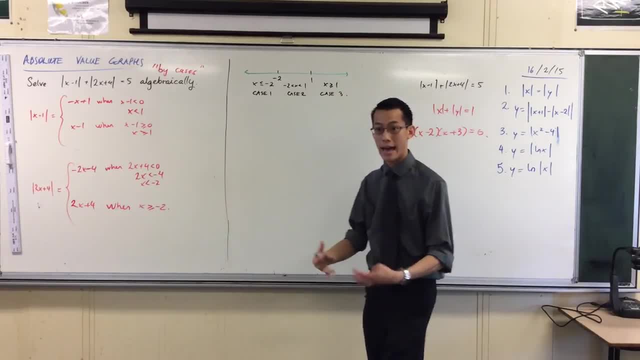 Okay, There are three cases, and now I just go through them one at a time. Right Case one. Okay, Now, when I said x is less than or equal to negative 2, which of these am I? I'm this one. 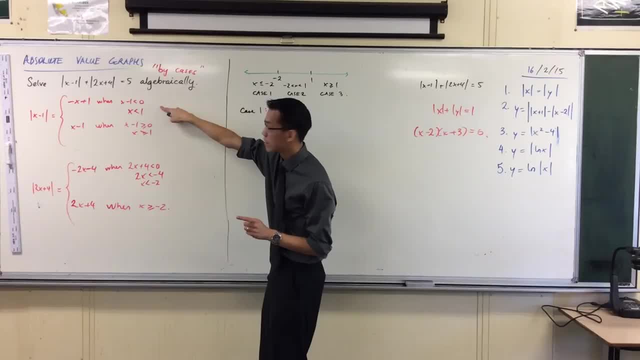 x is less than negative 2. Right, So therefore, yeah, that's right. Another way of thinking about this is they're both the negative case. So here's the first negative case and then here is the other negative case. 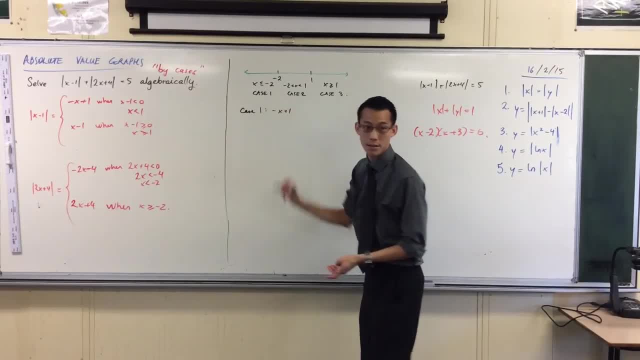 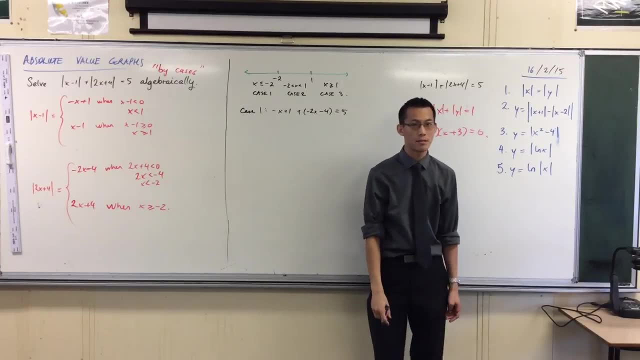 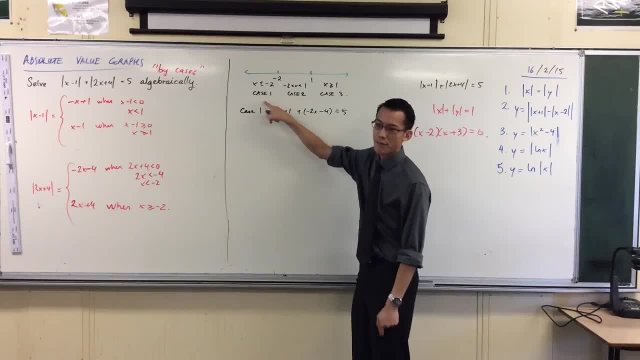 Yeah Yeah, Put the inside as well. Yeah, Yeah, I've justaut ogóle made sure that. so I'ma tell you what the må göster to tell. Yeah, I've just I've written that there, so that I'm gonna. so this is my diagram to tell. 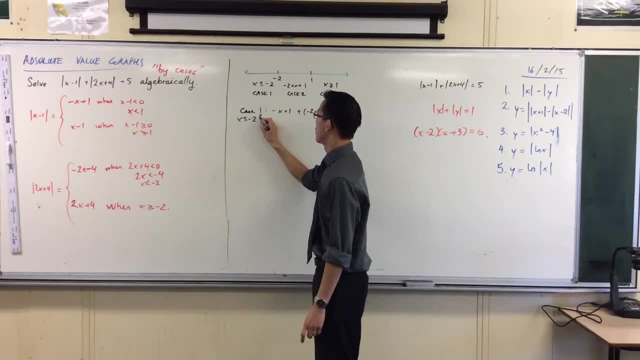 So I'm gonna. So this is my diagram to tell me what my cases are. Okay, I could write it again if you like. I should write it down to do a stew, interesante, Like. so You can take a slice of this. 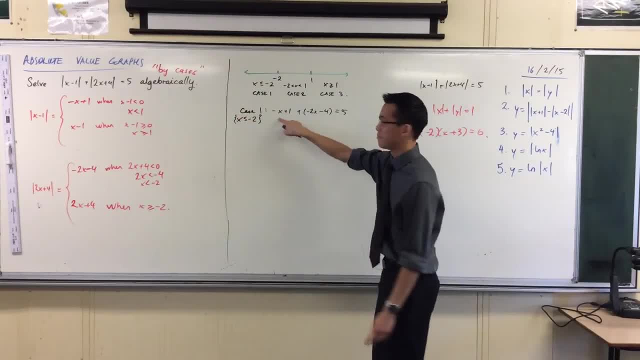 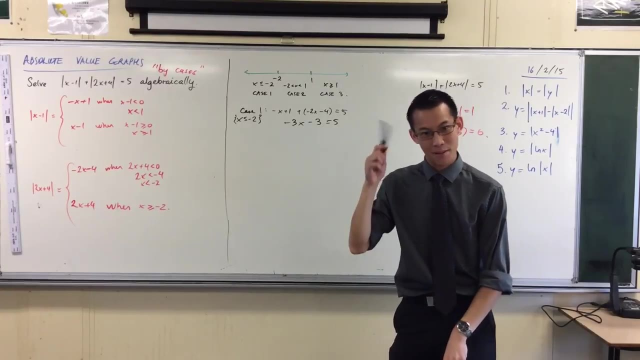 Okay, Help me solve it. Help me solve it. Collect some like terms over here for me. What am I gonna get? Hunch minus three, Minus Okay, year 11.. I've had a look and I've been listening as well, because my ears aren't that bad. 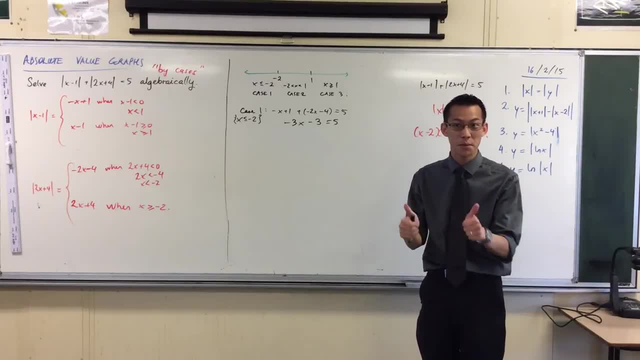 and I'm pretty sure all the conversations happening right now are good conversations and I want them to continue. I just want them to continue at a volume that lets the people who are trying to listen to this listen to it. Does that make sense? 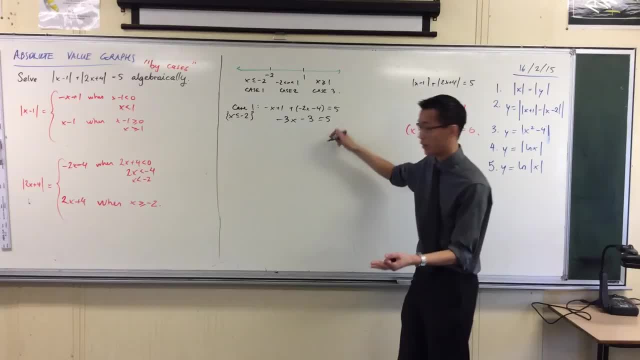 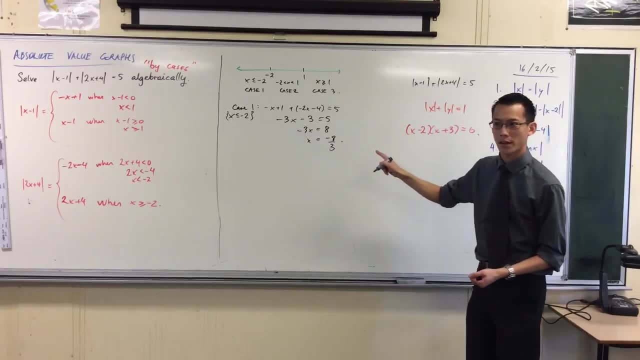 Cool, Let's keep going. All I'm doing over here is I'm just solving algebraic, which looks to me like that, which looks to me like this, which is a very familiar number. Okay, Now check that. Here's the important thing about cases, right? 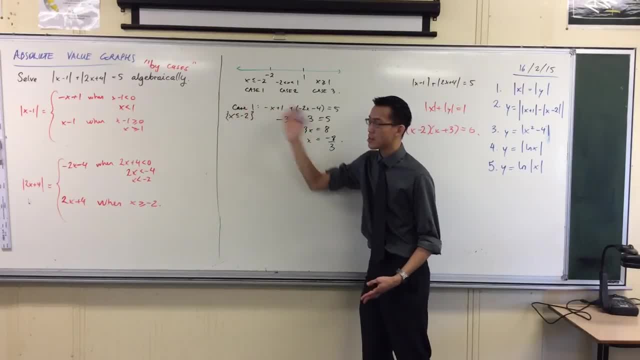 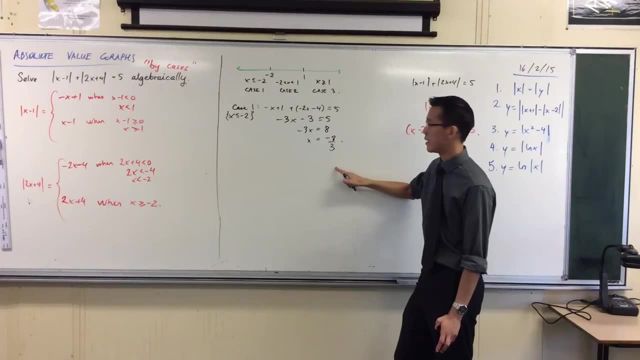 This thing is only true. this is what the absolute values are equal to. only where this is true, right? So you look at this and you say: does this lie within our restricted domain? Is is minus 2 and 2 thirds, is it less than or equal to negative 2?? And the answer is: 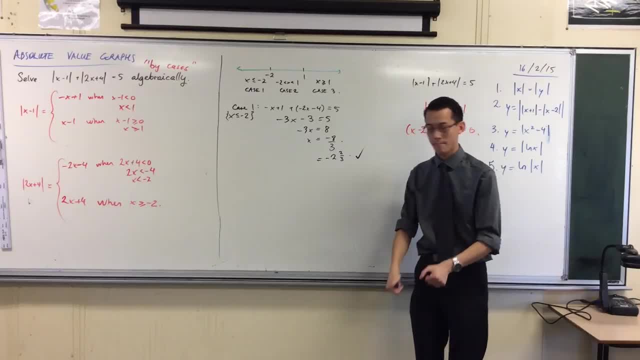 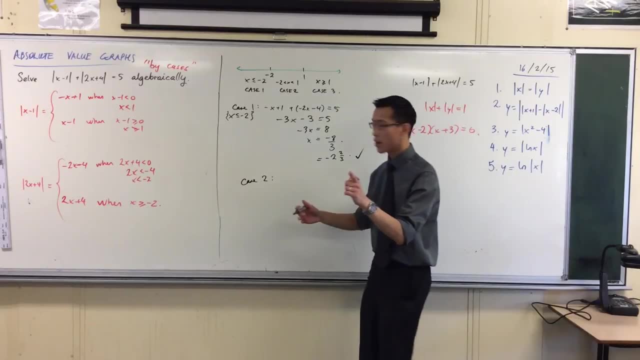 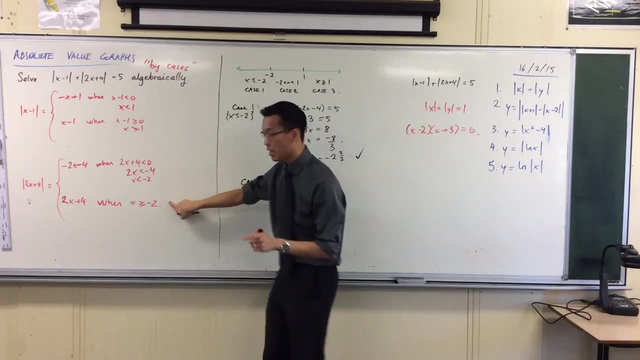 Yes, it is. So that's a solution. Thumbs up, Rinse and repeat Case 2.. Okay, You're going to put all the algebra together, but watch, Now I'm between here and here. right, So I am here. I'm greater than negative 2 now, but I've crossed over to whoops. what am I doing? 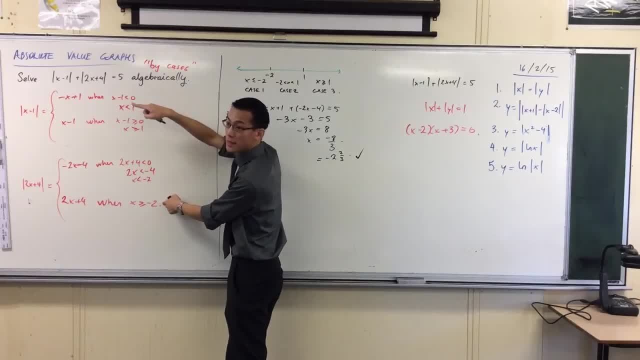 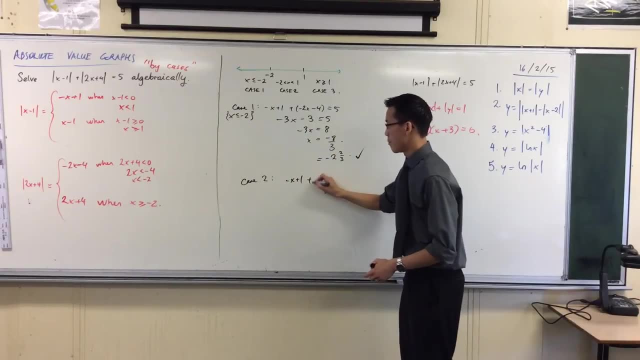 Still here. So this one's changed over to the positive case, but this one's still the negative case, Right? So case 2 will be negative. x plus 1, that one plus, and now I have crossed over to this one. 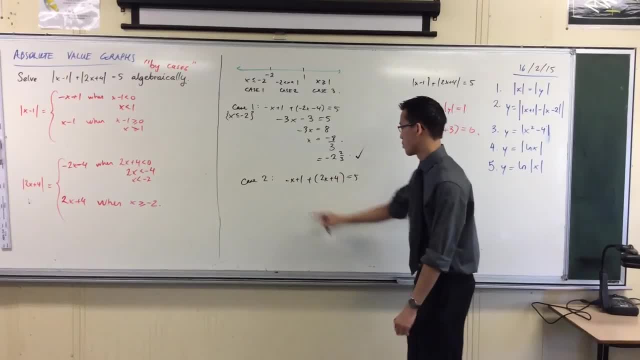 And that's equal to 5.. Okay, Again, you go through the algebra Here I'm going to get: x plus 5 equals 5, so x equals 0. You look at that, you check is the solution I've gotten. is it in my restricted domain? 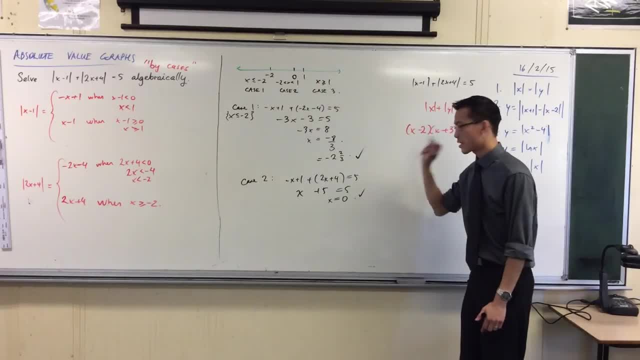 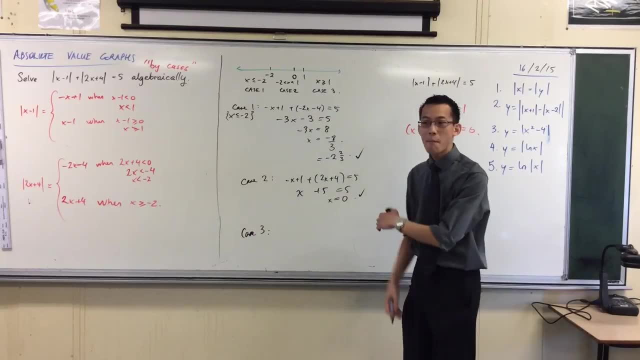 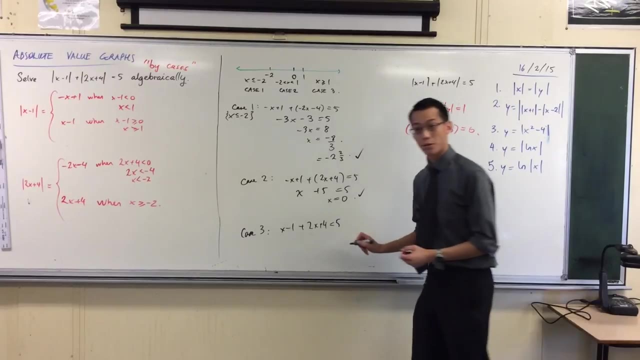 And the answer is Yes, it is Tick, It's a solution. Final case, Case 3.. Okay, Now, both of them are in the positive case, Right? So this is kind of easy to write. I just say x minus 1,, 2x plus 4, that's equal to 5.. 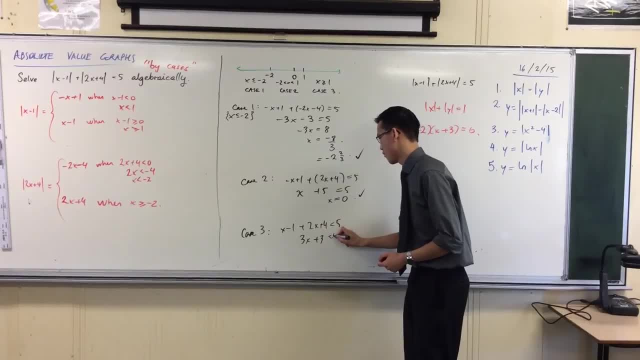 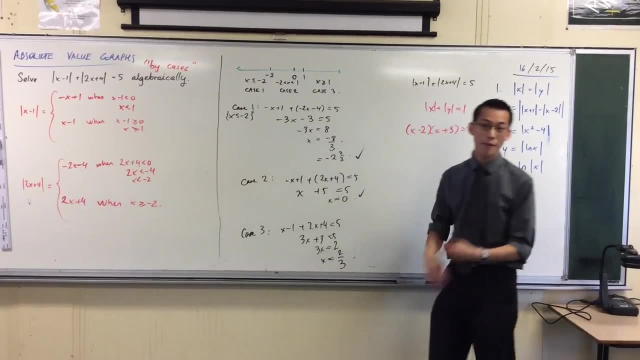 3x, let's see 3,, 5,. take that over to that side. you divide through and, just like we have with all the other cases, you look at this and you say: is this within the restricted domain that I've defined? 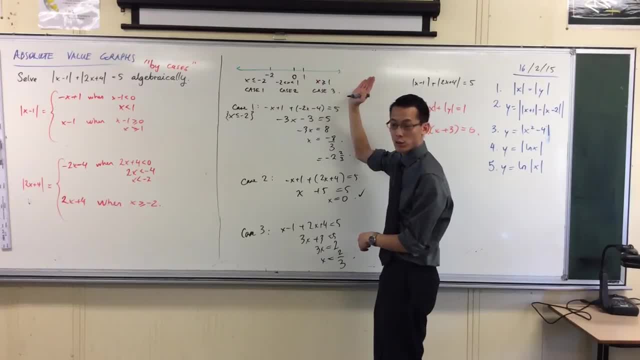 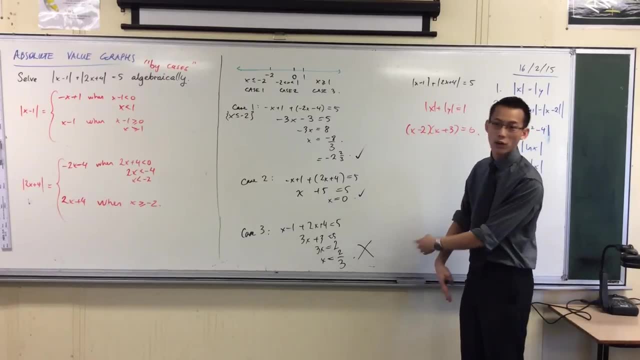 And you say, uh-oh, I'm not. I should be greater than or equal to 1, but this is not. So this is not a solution. This is an extraneous solution, Right. So now I've gone through all my cases, I've worked out which solutions are valid and which ones aren't. 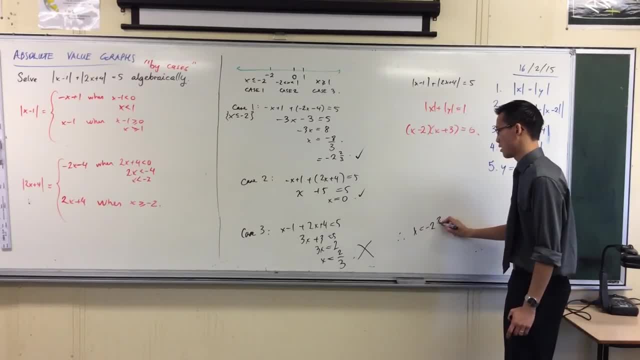 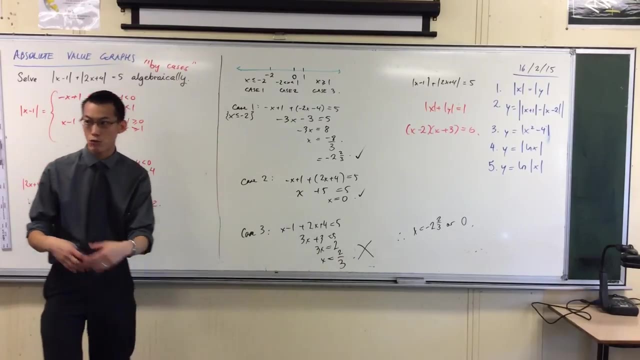 and so I say, therefore, x is negative 2 and 2 thirds or 0, and that's it. So I'm not a huge fan of this right. It's a very blunt tool, because you can't know which cases are going to be right or not until you get to the very end of solving the algebra. 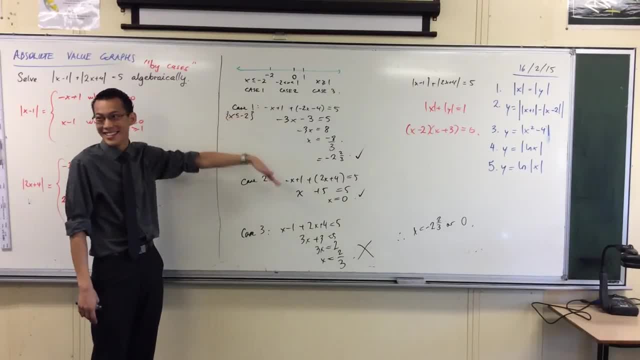 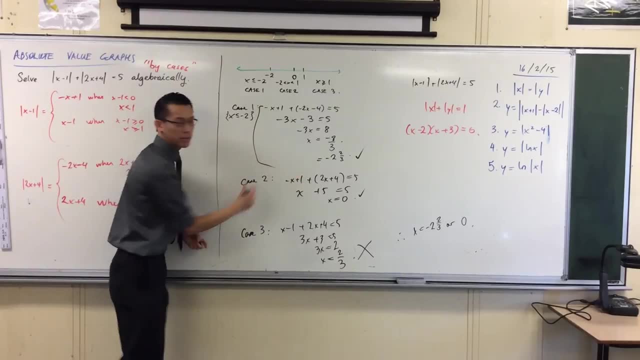 Right, Which, by the way, this is not too bad in the scheme of things. It can get a lot messier than this. So can you imagine going through 1, 2,, 3,, 4,, 5,, 5 plus lines of working that are taking you time?